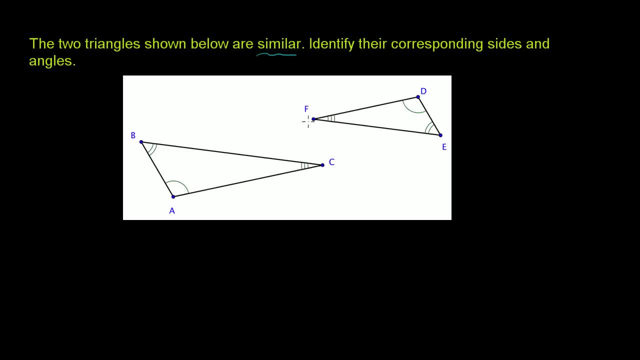 And this angle over here with three arcs is equal to this angle with three arcs over there. So that's how we can identify which angles correspond to which other ones. So, for example, angle CAB corresponds to this angle over here which we can call FDE. 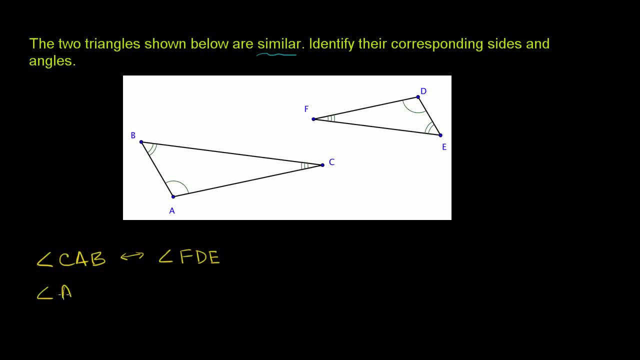 If we say angle ABC, this corresponds. So now we're looking at this angle right over here. Angle ABC corresponds to angle DEF, And then finally, angle BCA, which is that angle over there we look at the three bars, corresponds to angle EFD. 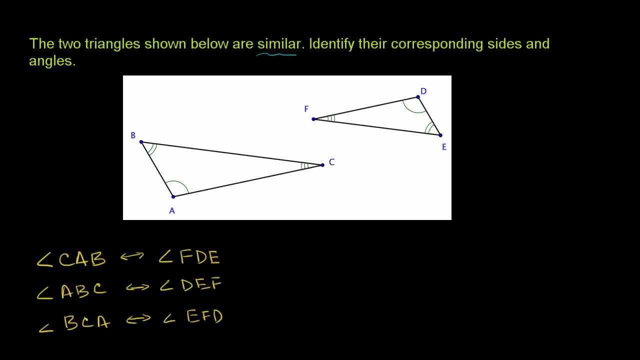 Now, when we think about corresponding sides- and let me color code it- actually That'll make it a little bit more interesting- Side AB, so let's say side AB, segment AB, I guess you could call it. corresponds to what? 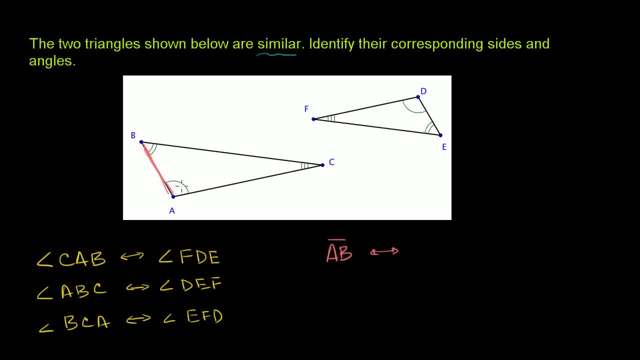 Well, you can tell by looking at the angles. This is the side between this one arc angle and this two arc angle, the side between the one arc angle and the two arc angle. It corresponds to side DE on this triangle, the segment DE. 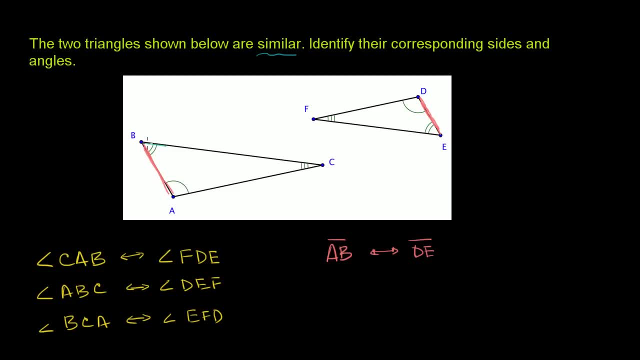 Then if we look at BC right over here, BC corresponds to: it's between the two bars and the three bars, between the two bars and the three bars, It corresponds to EF. Another way that you could think about it is that this blue side. 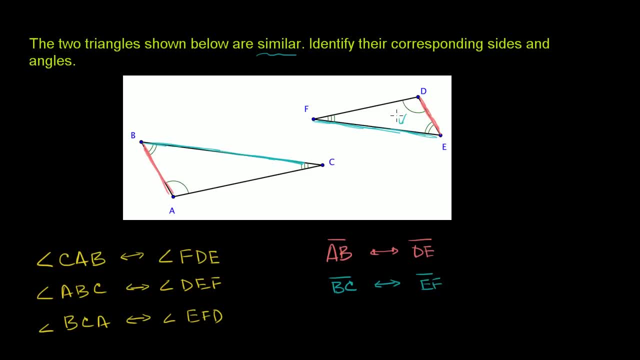 is opposite this angle: EDF or FDE. we called it Well, we called it EF. It's opposite FDE. over here It's opposite an angle and it's opposite this angle, the one arc angle, This orange side, was opposite the three arc angle. 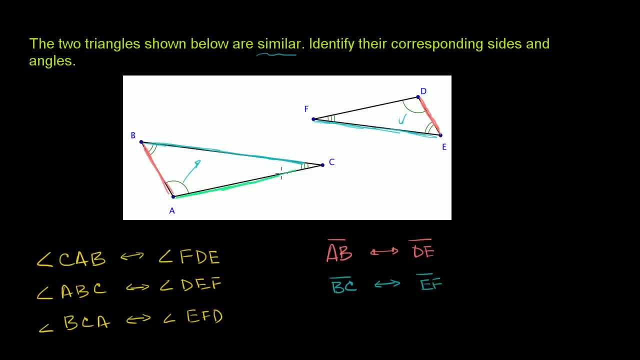 And then, finally, if we look at this side, right over here, AC, it corresponds to- well, it's the only one that's left, but it's also AC is opposite that two bar angle. It is right over here. It corresponds to side DE.